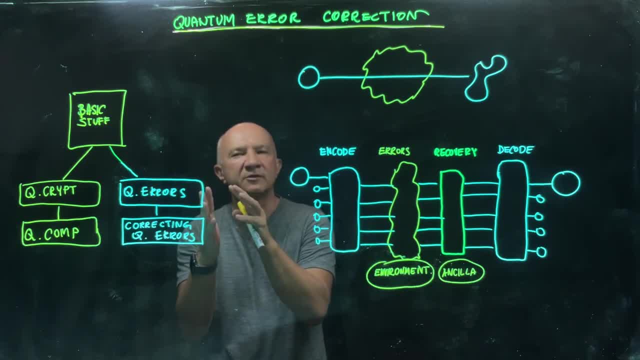 approaches here right. So you can think about a unitary evolution of the whole when you include the environment, That's the so-called Stein spring representation. But you can also look at the system alone and ask the question: what is the unitary evolution of the whole? What is the unitary evolution? 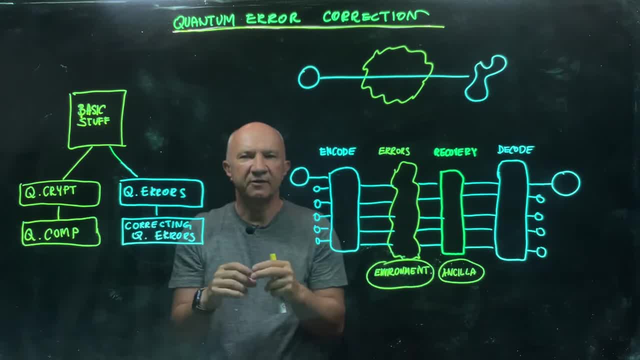 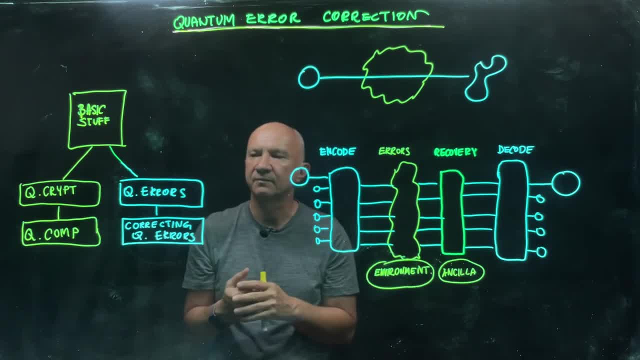 of the environment, but not necessarily just including the environment in your equation. So that's the Krauss representation. Now we have the tools, so we can now move on and discuss how we can deal with quantum errors. So whenever, remember we call Krauss operators quantum errors. 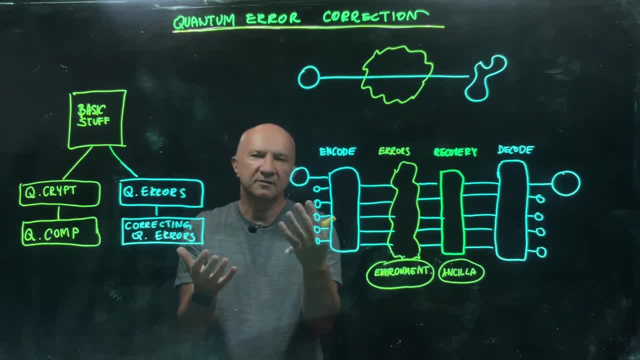 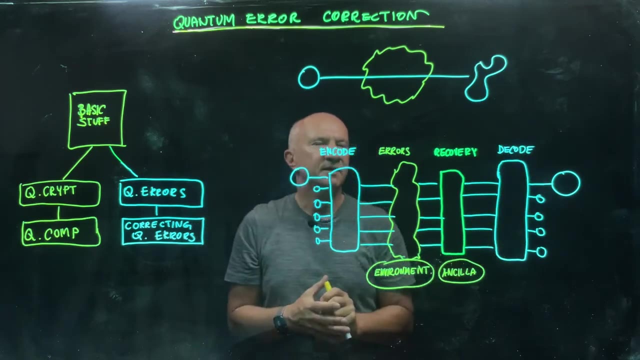 The question really is: given a system that undergoes some sort of evolution, described by a completely positive map, is it possible to recover the original state of the system? So I would like you to have this kind of scenario in mind. So compare the two cases. 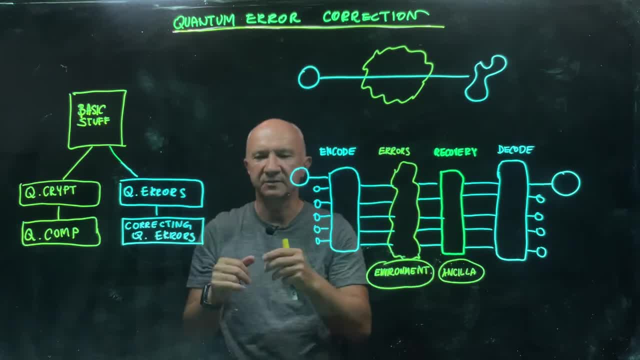 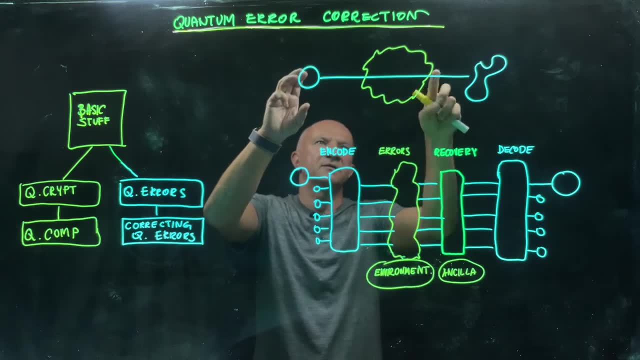 The case where we have a system, let's say it's a qubit. you can always choose the simplest possible quantum system, So we have a qubit. This qubit undergoes decoherence, so interacts with the environment And, as a result, the state of the qubit is. 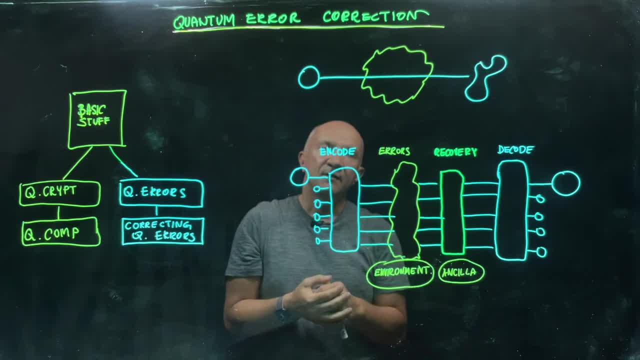 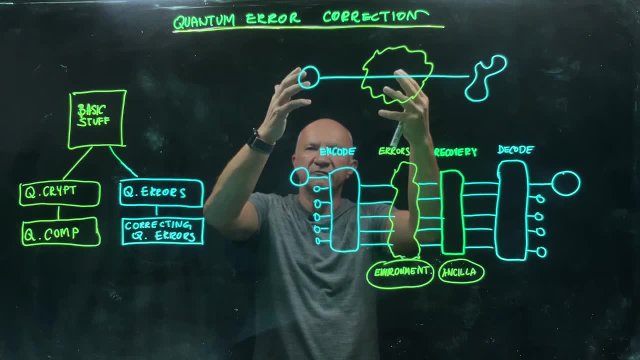 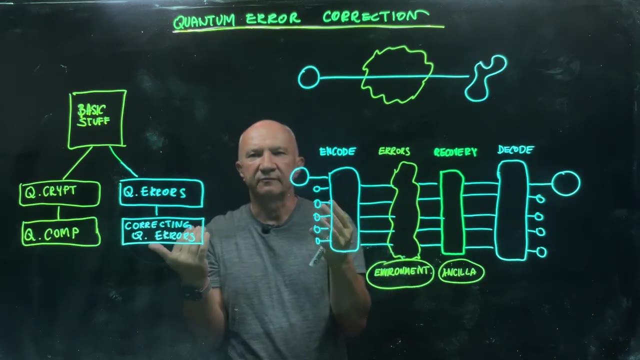 modified in some way? Now is there a way to diminish the impact of the environment? And here we are going to borrow ideas from classical theory of information. So we are going to use the concept of error correcting codes. So, instead of this kind of scenario, we are going to encode the 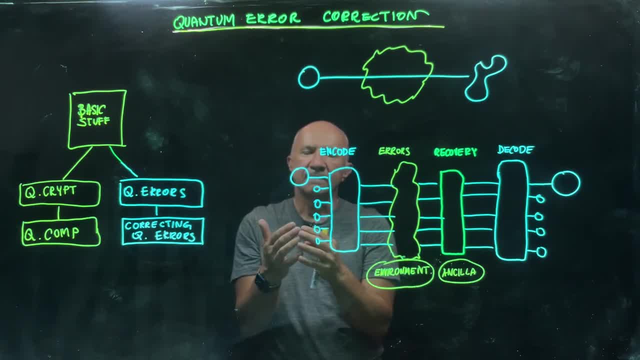 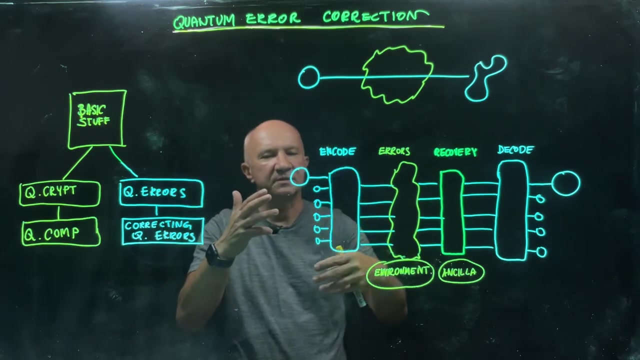 state of the qubit into a number of qubits. So we are going to bring a few more qubits and take our original qubit and we are going to perform a unitary operation that maps unknown state of the qubit into a set of qubits that will form our encoded qubit. 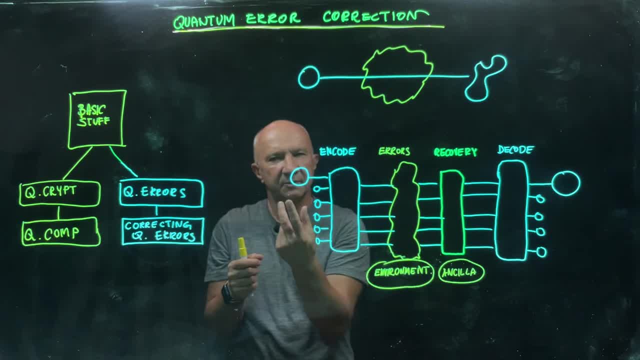 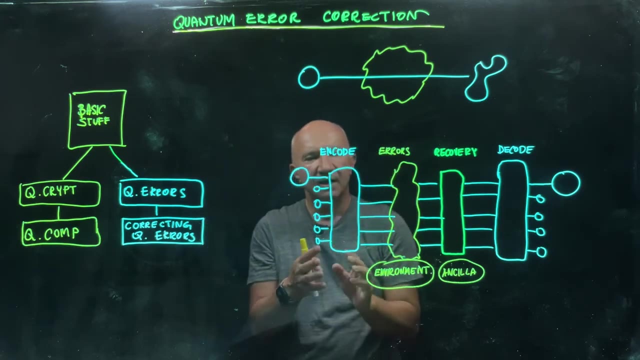 So this, mathematically speaking, we are just going to pick up a two-dimensional Hilbert space and we are going to embed it in a higher-dimensional Hilbert space, rotate somehow. That's isometry, right? So that's going to be the encoding part. 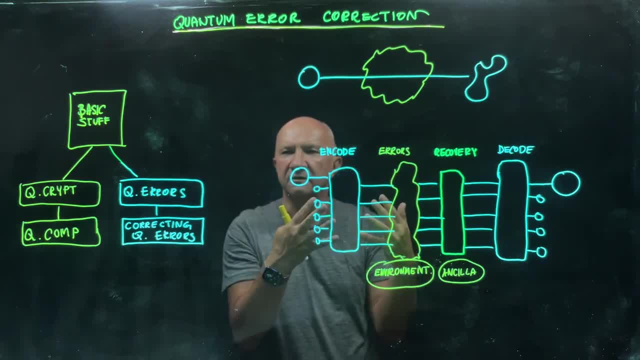 And then all the qubits go to the decoherence area, So errors will appear. And then, at this point you may be a little bit confused. And then, at this point you may be a little bit confused, You say okay. well, now the errors will appear on many qubits. 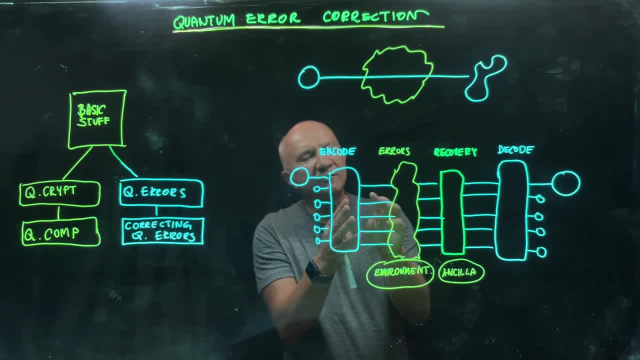 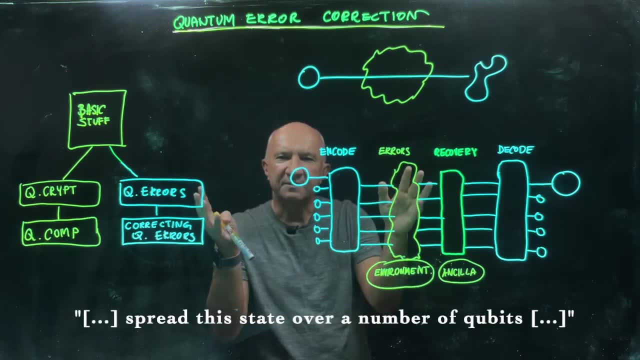 Well, yes, but if you just take the quantum state of one qubit and somehow spread the state know of qubits, Know of qubits, Know of qubits, the error on one qubit may not perhaps be so significant. It may be possible to recover. 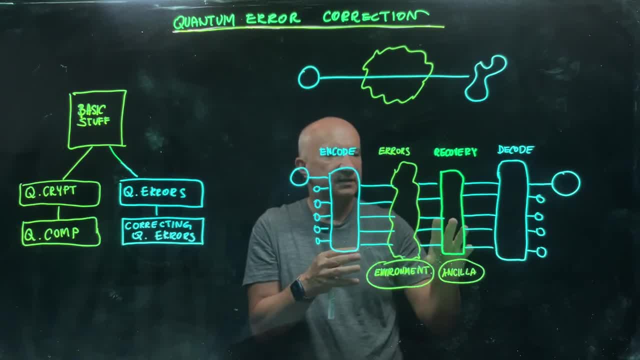 it under certain conditions, And indeed we will see that under certain conditions, it is possible to recover, to reverse this completely positive map. So the first one: the errors are induced by the environment, which you cannot control, But as long as you can find. 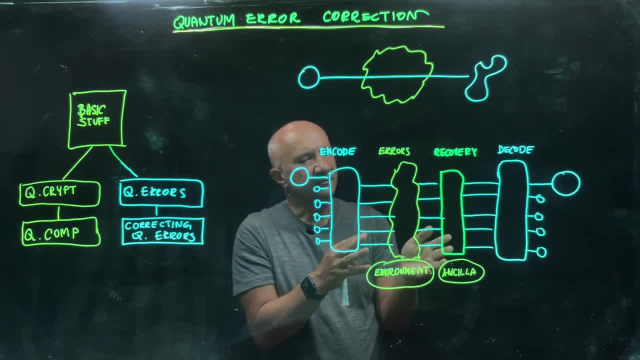 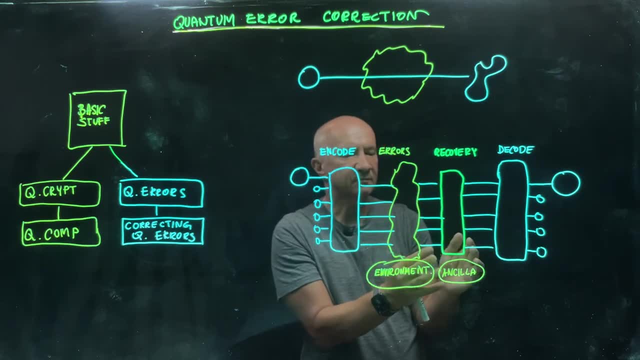 out roughly what happened then you can then just apply another, completely positive map. In this case we don't have the environment, but we just bring extra even more qubits or some other quantum systems, auxiliary qubits or a system that we call Ancilla, a kind of 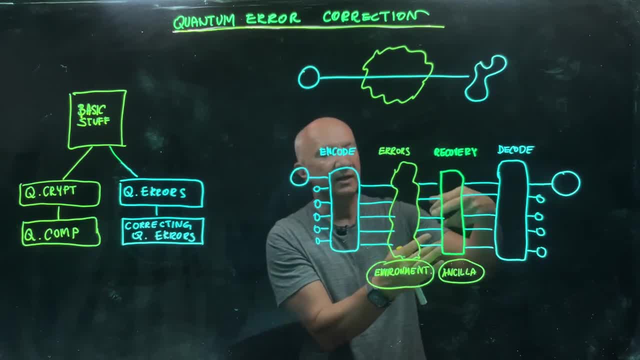 helper to help us to perform in a controlled way another completely positive map. So that's going to be error recovery And then Once, Once hopefully- we manage to recover the original state of all those qubits. then we just simply decode the quantum state, So we just map the state into the qubit and hopefully 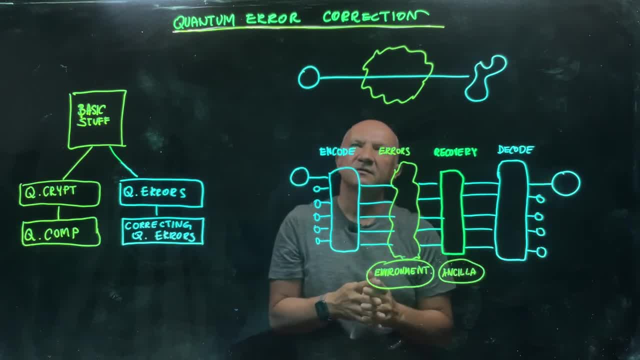 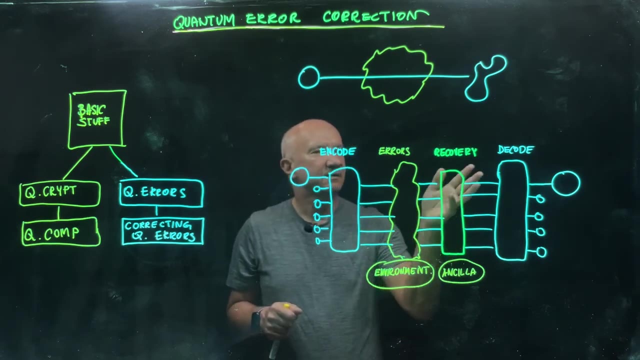 we'll have something that is very close to the original. So I would like you to have this scenario in mind And, of course, you know, in the lecture we will go through all the details and I'm going to tell you how to encode, how to construct the recovery procedure.